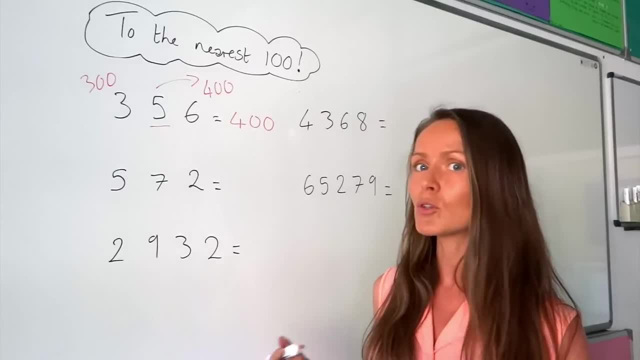 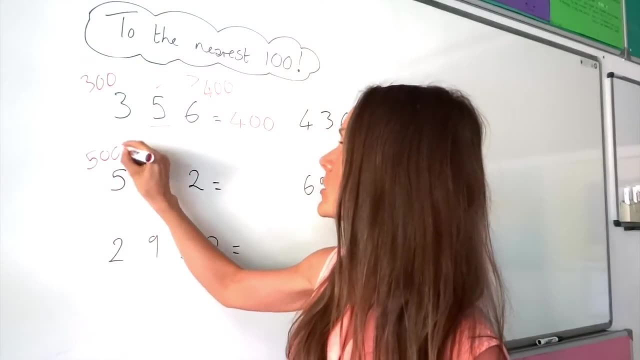 the same way, and I'm just going to jot down the two multiples of 100.. One that's smaller than this one and one that's bigger, So I've got 500 and 600.. Okay, so these are the multiples of 100 that. 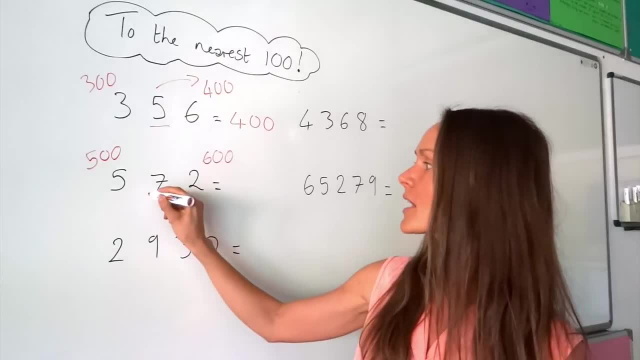 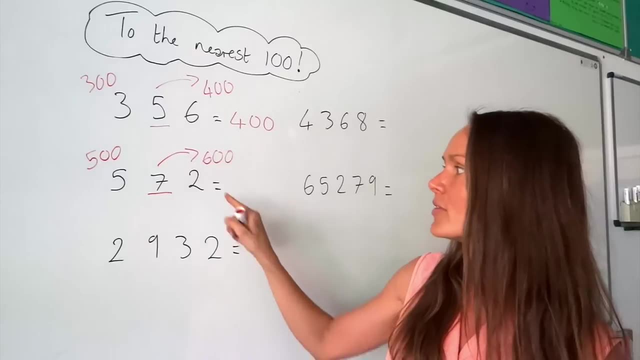 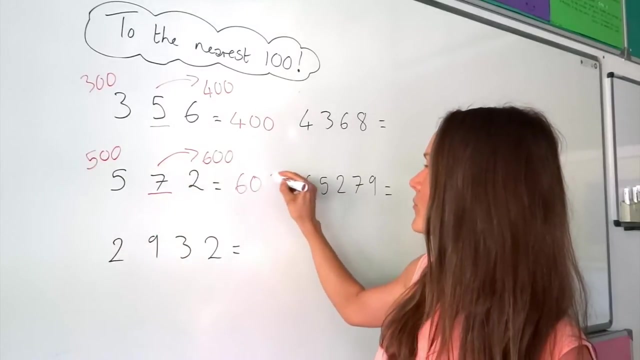 I'm going to write down on either side of the number. So, because the second from last digit is seven, that means we have to round up, But you can probably see already that this number is closer to 600 than it is to a 500.. Okay, so there's that one. All right, this one down here. So the number's. 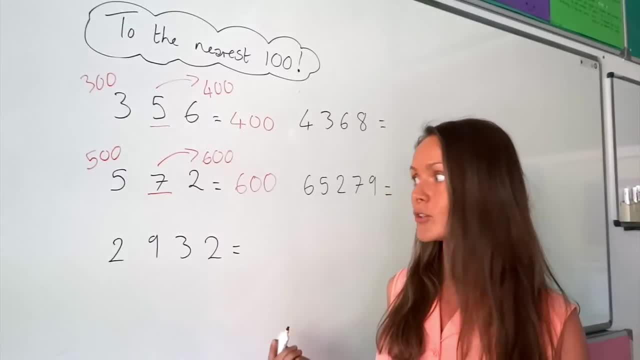 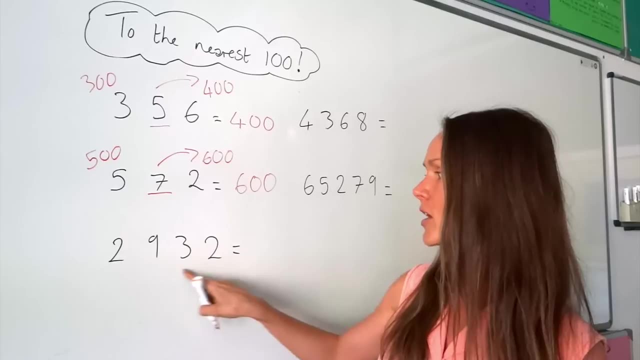 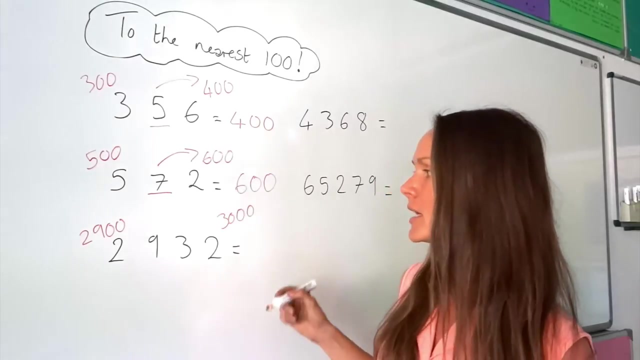 getting bigger. but that's fine, It's exactly the same method as before. So I'm going to write down the full either side of this number. So I've got 2,900 and I've got 3,000.. Now, if you can't see, 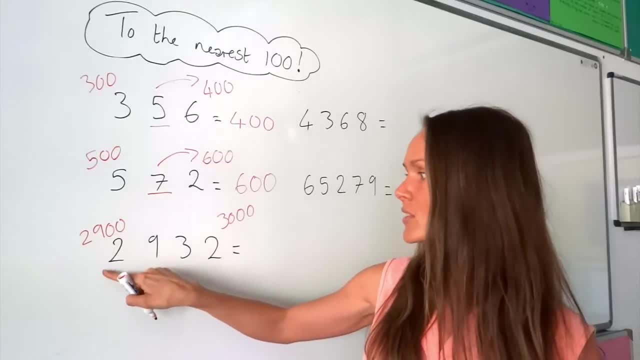 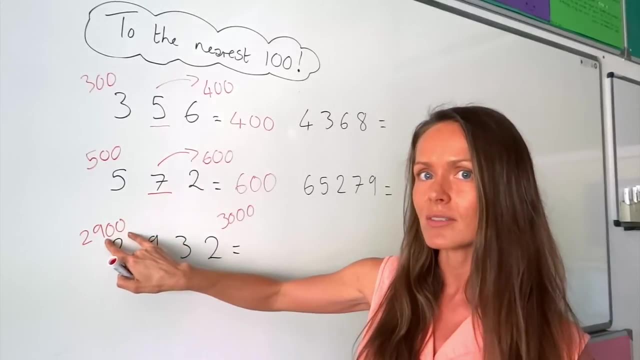 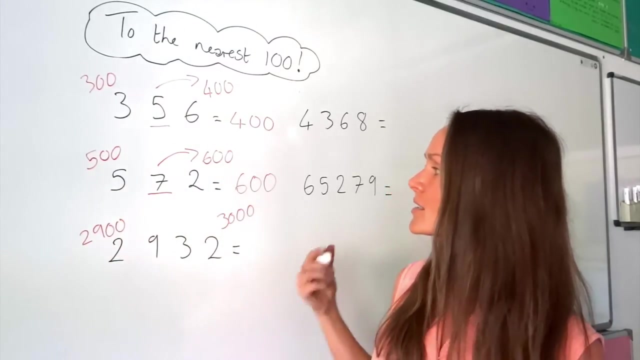 where I got those numbers from. the smaller number is just this number written out again, but we're replacing the last two digits here with two zeros, And this number here we can find by adding 100 to this number on the left. Okay, so, just like before check the second from last. 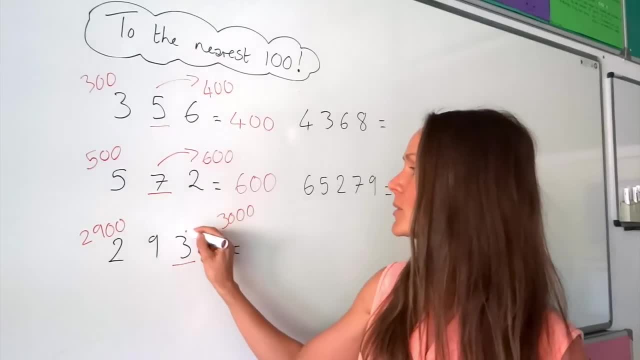 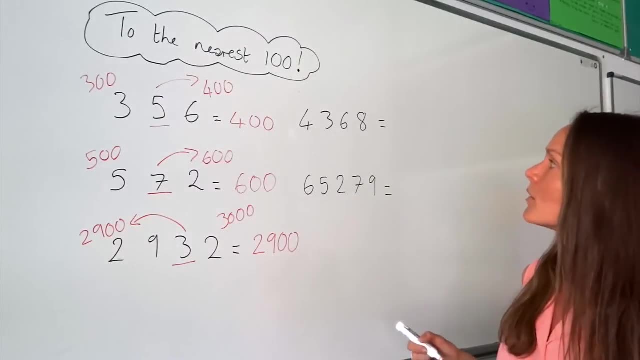 digit number, And this time it's smaller than five. So that means we need to round down. So the answer is 2,900.. And I'm going to do the same with this one up here. I'm going to write down my 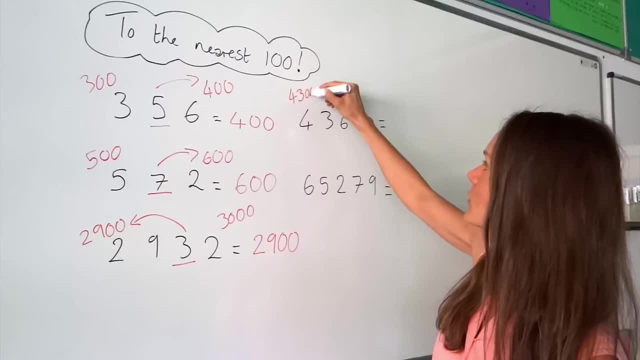 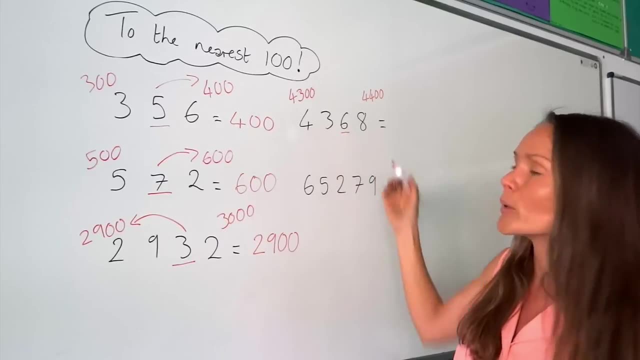 multiples of 100,: this one which is smaller than the number and this one which is bigger than the number. And because the second from last digit is bigger than five, that means I have to round up Okay, and the last one, So an even bigger number. but it's exactly the same method as in these other 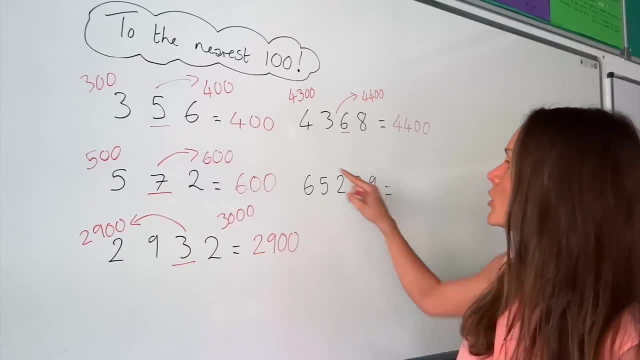 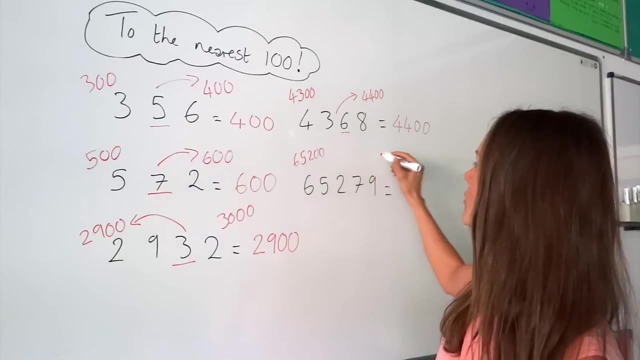 examples here. So I'm going to start by writing down the two multiples of 100 either side of this number. So I've got 65200 and 65300.. Remember, if you can't find these, if you don't know what, 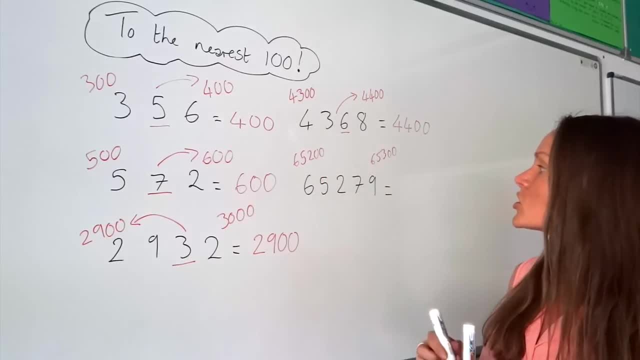 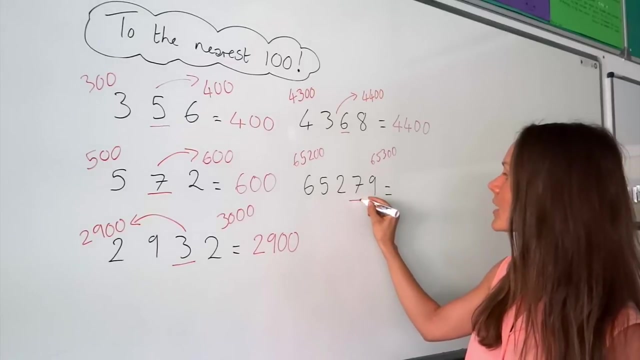 these multiples of 100 are either side of the number. just write that number out again, but replace the last two digits here with two zeros, And then, to find the bigger one, you just add 100 to this number here. So just like before, check the second from last digit. 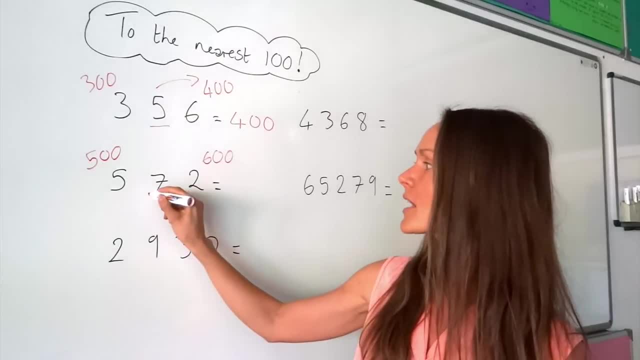 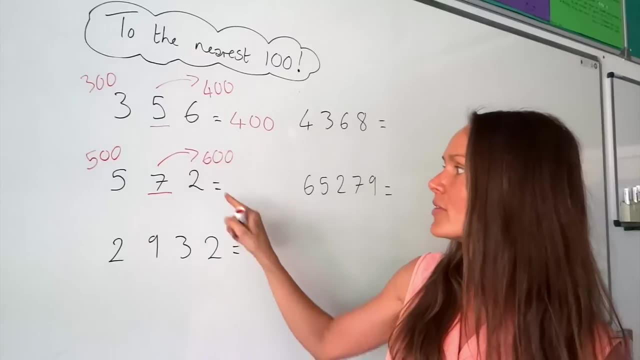 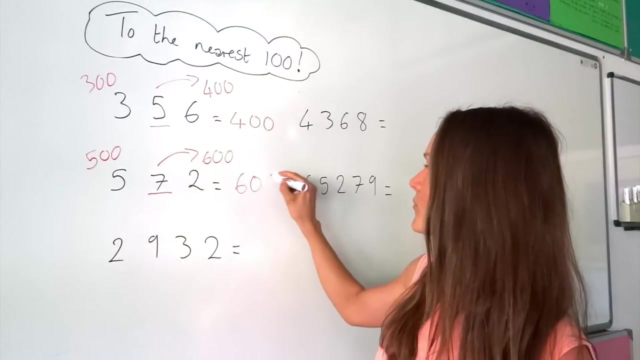 are on either side of the number. So, because the second from last digit is seven, that means we have to round up, But you can probably see already that this number is closer to 600 than it is to a 500.. Okay, so there's that one. All right, this one down here. So the number's getting bigger. 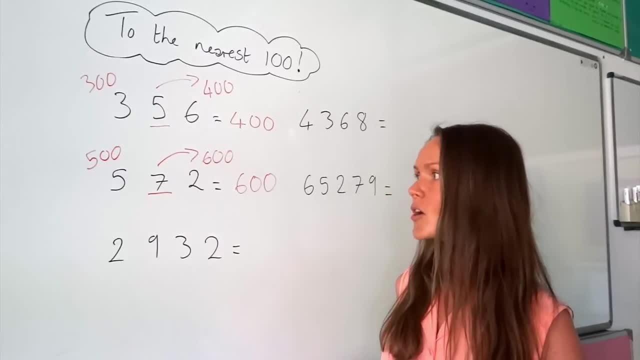 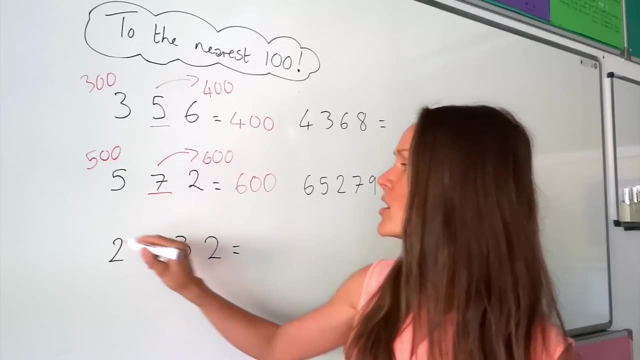 but that's fine. It's exactly the same method as before. So I'm going to write down the two that fall either side of this number. So I've got 2,900 and I've got 3,000.. Now, if you can't see, 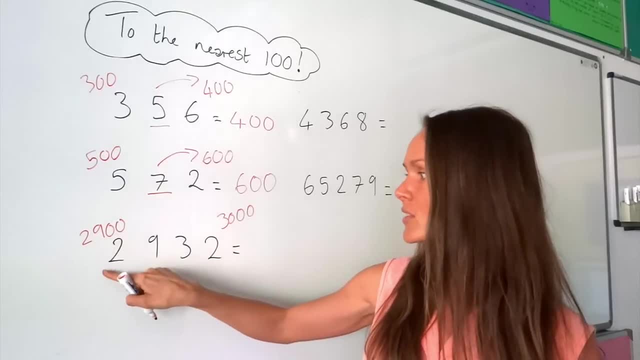 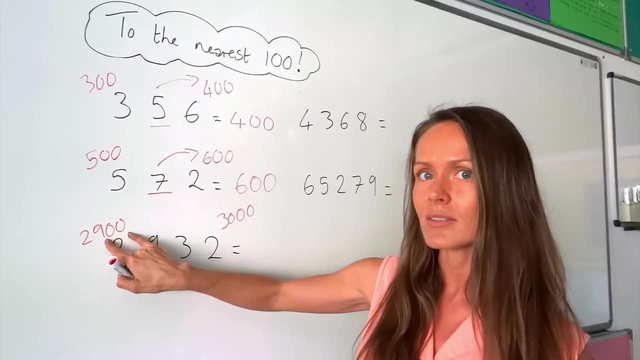 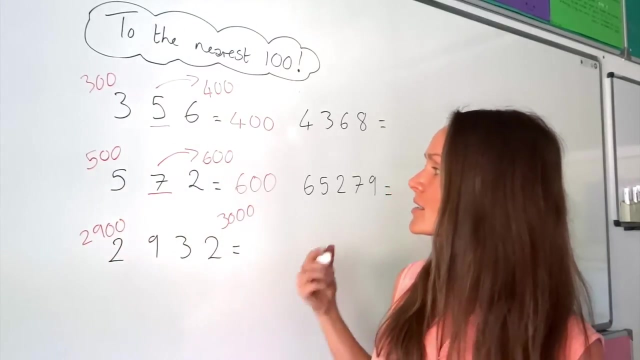 where I got those numbers from. the smaller number is just this number written out again, but we're replacing the last two digits here with two zeros, And this number here we can find by adding 100 to this number on the left. Okay, so, just like before check the second from last digit. 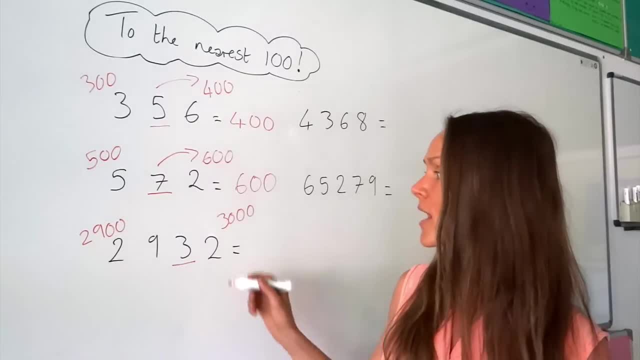 in your number. So I've got 2,900 and I've got 3,000.. Now, if you can't see where I got those numbers from, and this time it's smaller than five. So that means we need to round down. So the answer is: 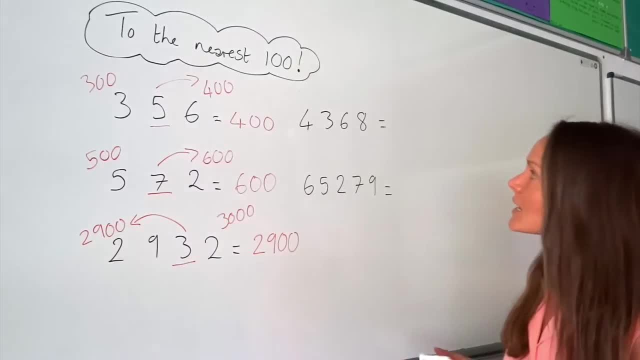 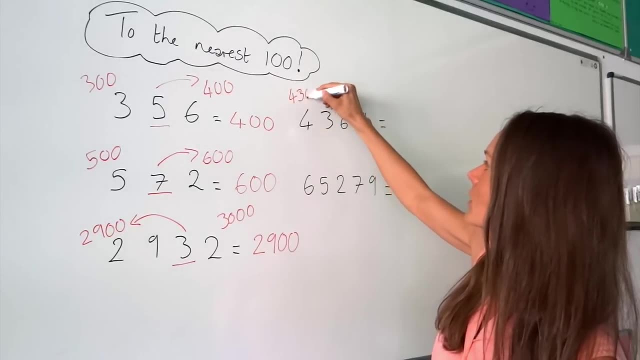 2,900.. And I'm going to do the same with this one up here. I'm going to write down my multiples of 100, this one which is smaller than the number and this one which is bigger than the number. 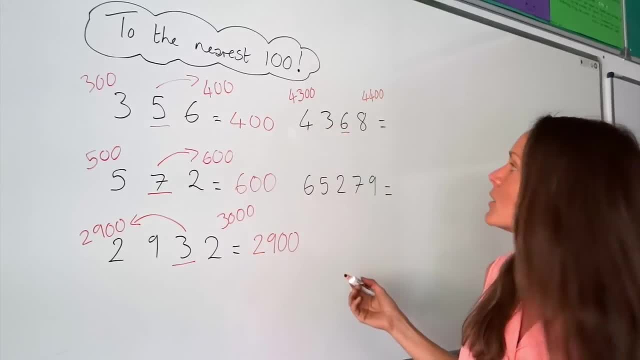 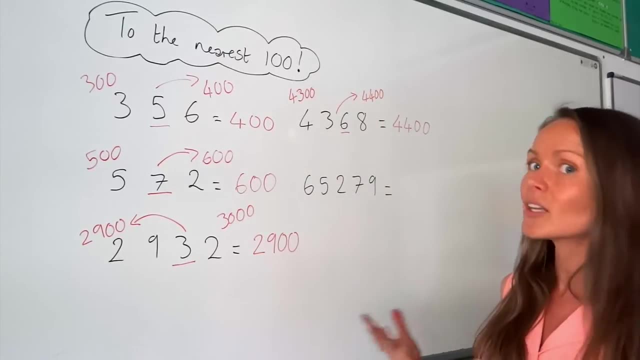 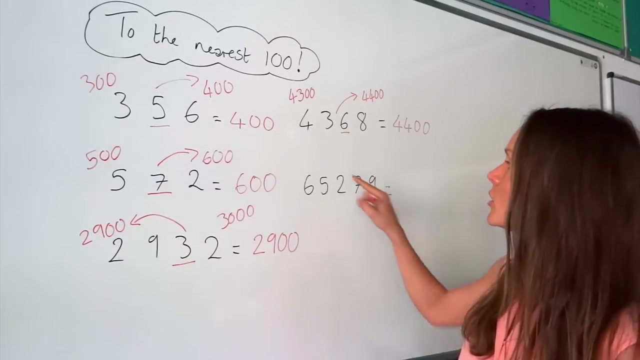 And because the second from last digit is bigger than five, that means I have to round up, Okay, and the last one, So an even bigger number. but it's exactly the same method as in these other examples here. So I'm going to start by writing down the two multiples of 100, either side of 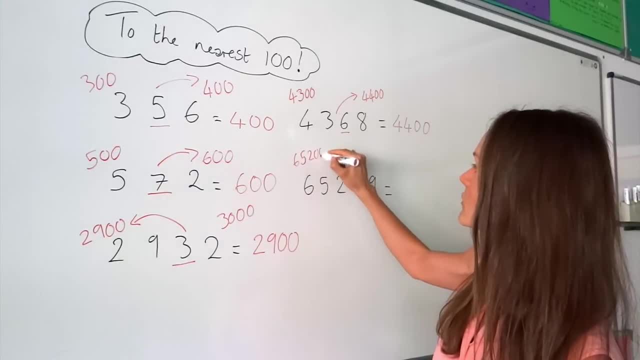 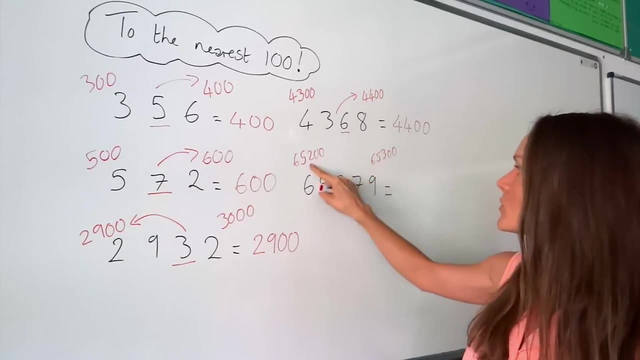 this number. So I've got 6,5200 and 6,5300.. Remember, if you can't find these, if you don't know what these multiples of 100 are either side of the number, just write that number out again. 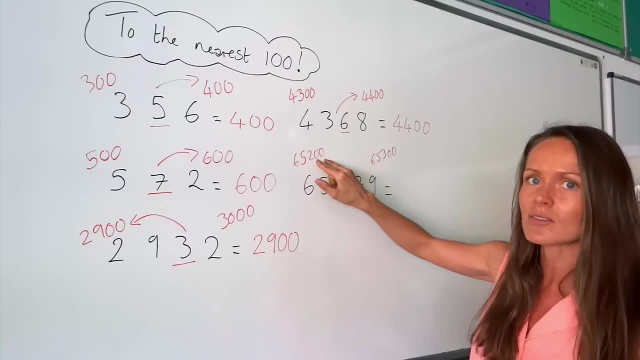 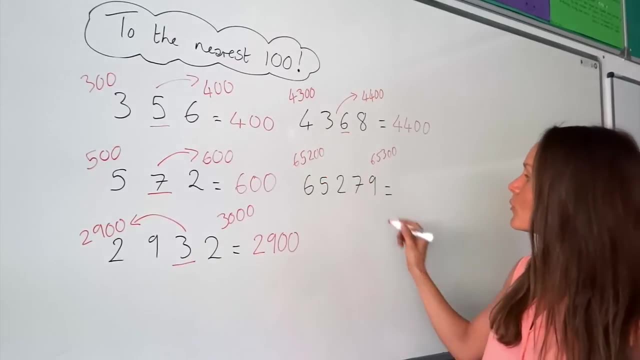 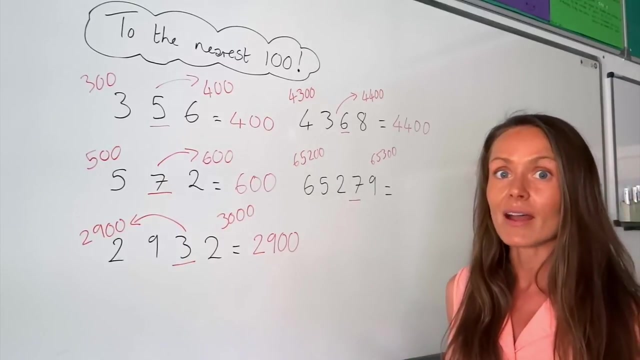 but replace the last two digits here with two zeros, And then, to find the bigger one, you just add 100 to this number here. So, just like before, check the second from last digit in your number. And because this one is larger than five, that means we have to round up.